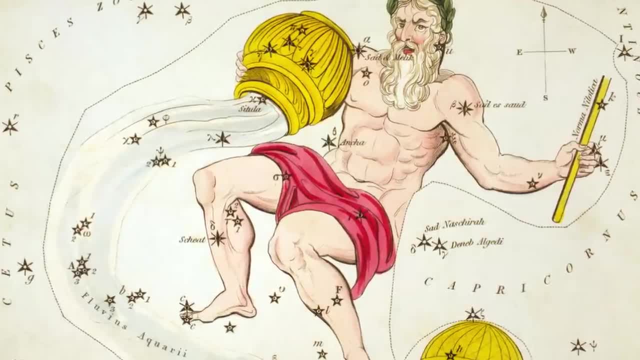 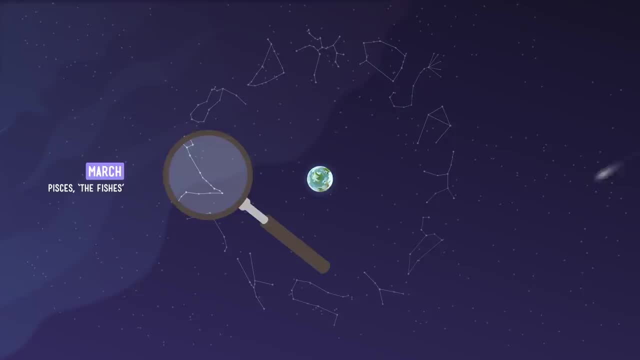 called the Babylonians thought that this group of stars looked like an old man pouring water from a pitcher. Moving on to March, this is Pisces, or the fishes. Pisces represents Venus, a Roman goddess who is said to have turned into a fish and jumped into a river to escape. 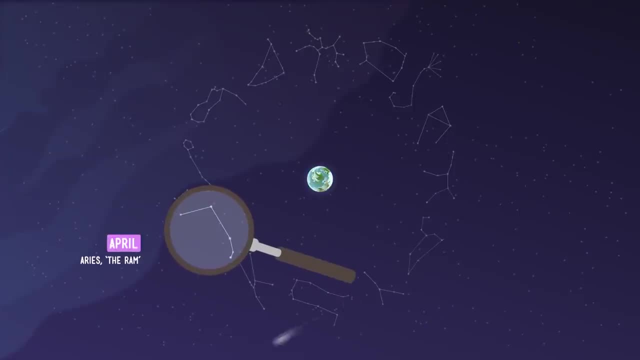 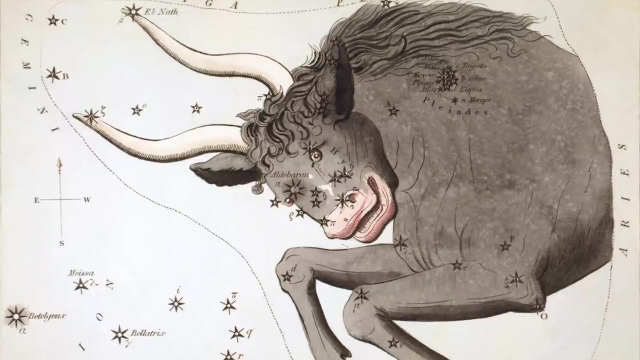 an evil monster. Aries is up in April. In Greek mythology, Aries was a ram with wings. The constellation of Taurus, visible in May, looks like a bull. It's named for the Roman god, Jupiter, who could supposedly turn himself into a bull when he swam. June's prominent 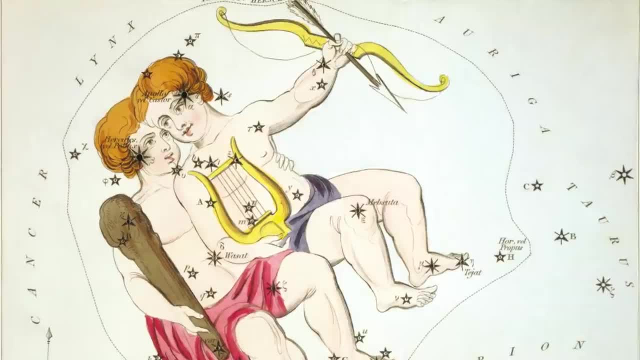 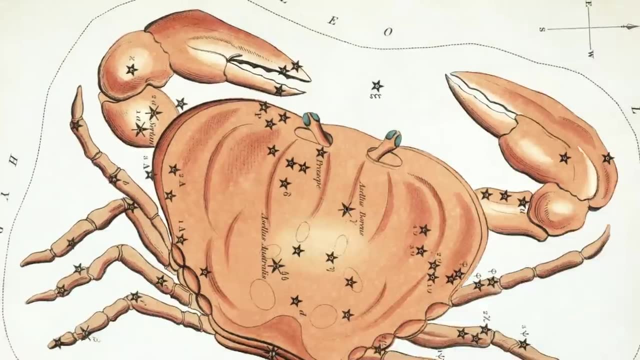 constellation Gemini is sometimes called the twins, because it reminded the ancient Greeks of the twin sons of Zeus. Cancer, which you can see pretty well in July, is called the crab, because that's what it reminded some folks of. August's constellation is called 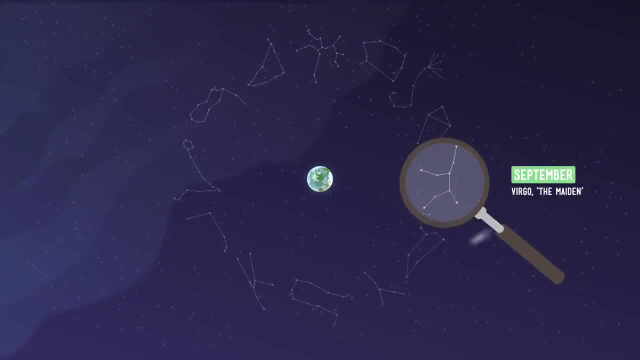 Leo and looks like a ferocious lion Seen in September. Virgo is called the maiden, since it looks like a lady holding grain, which symbolized the harvest to the Greeks and the Romans. The constellation of Libra appears in October, when days and nights are roughly equal and 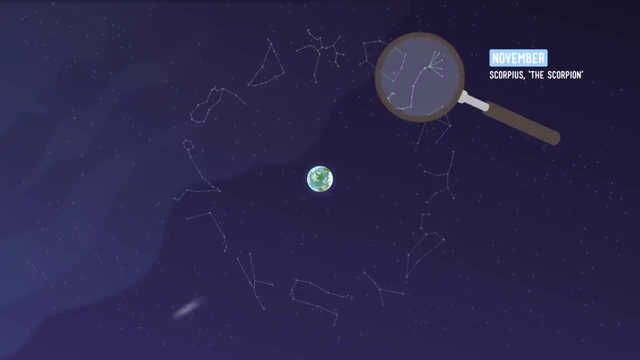 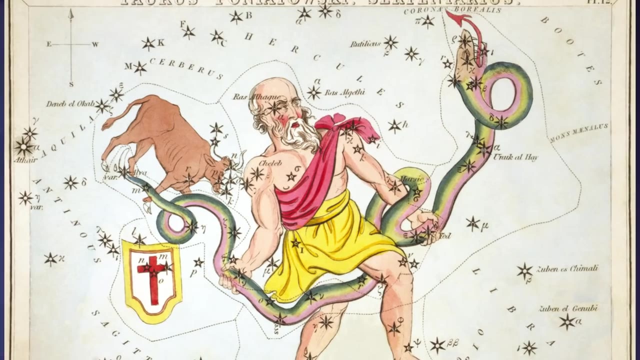 is considered a symbol of balance. I bet you can guess what Scorpius is named for. Yep, it looks like a scorpion Finishing off the year in late November is Ophiuchus, which was once called Serpentarius because it looked like a man holding a serpent or a snake. Hey, 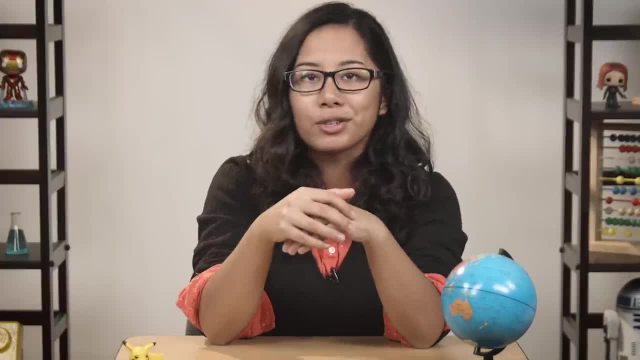 better him than me All. right, now that you've met all of the constellations in the zodiac, let's light them up and see if we can spot a pattern. Looks like a circle to me, And here's a fun fact. 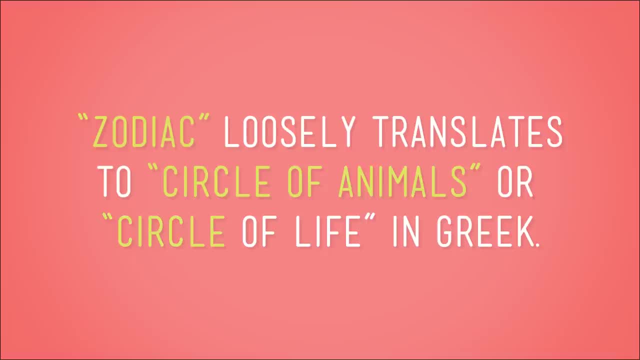 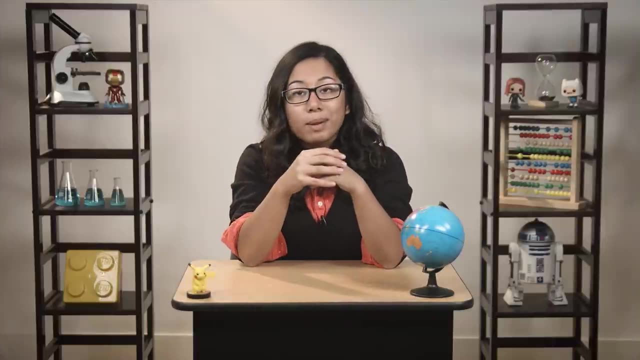 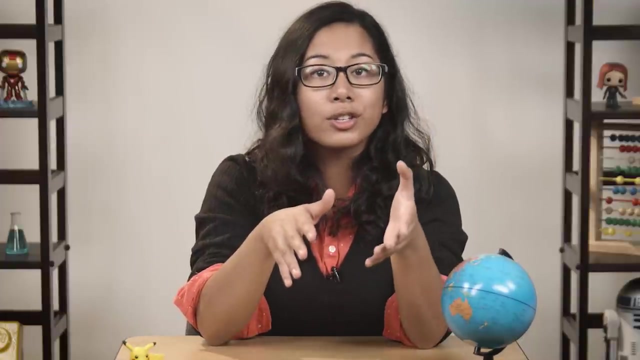 Zodiac loosely translates to serpent. Zodiac is a circle of animals, or circle of life in Greek. So the zodiac isn't just a random bunch of stars. It's a group of constellations that form a circular pattern in the night sky. And now you know which constellations are. 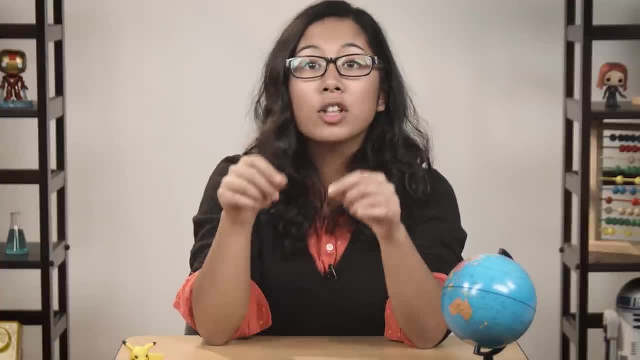 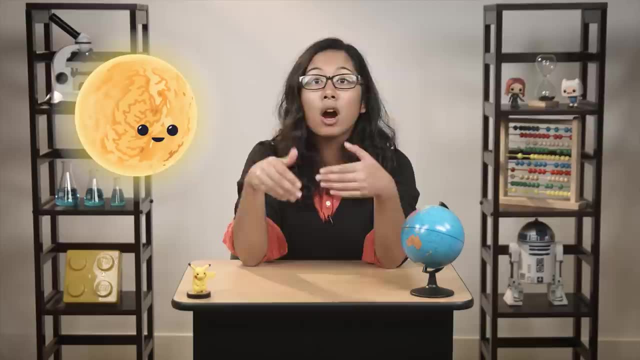 part of this pattern and that people have been observing these constellations for centuries. The zodiac has helped astronomers figure out how other objects travel in space- objects like the sun and even our own planet- But you can look forward to learning more on that. in the next episode.